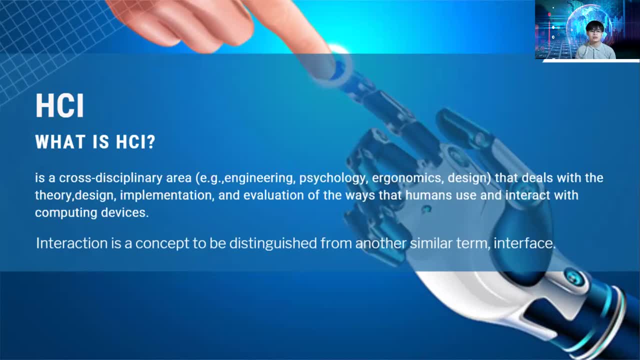 deals with a theory, falou, husband valenta, nature, logic and the science that you know: design, implementation and evolution of the ways that human use and interact with computing devices. So human-computer interaction is basically focused. it's 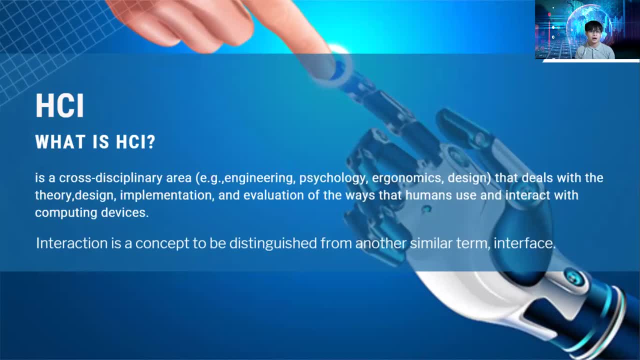 mainly focused on the interface between the user, or you, and the computing devices. So it evaluates of the ways that human use and interact with computing devices. from the terms itself, the human-computer interaction. It is how we interact with computing devices. So it is expected that by the end of this, 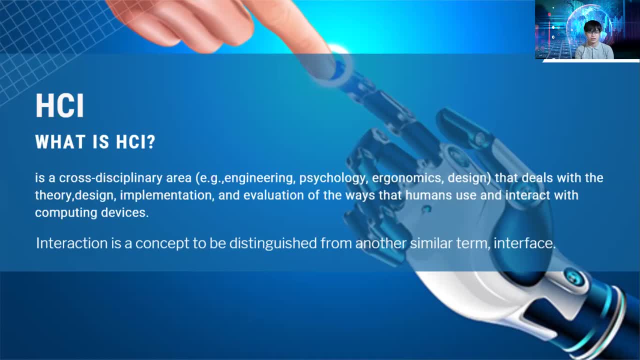 semester, since human-computer interaction. it involves interaction interface. you will be able to create and design your own application or your own system. okay, And it is. the interaction is a concept to be distinguished from another similar term: interface. So when we interact to a computing devices, there is 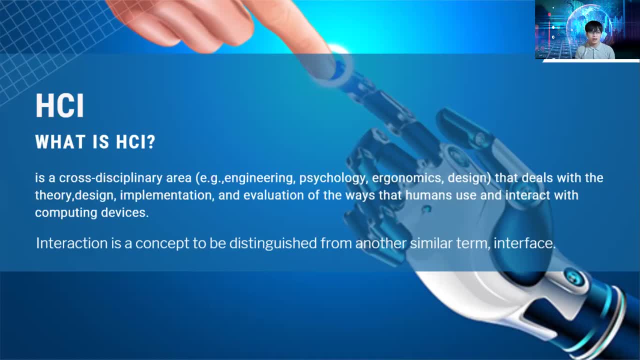 always an interface, right, Because it would be very hard for us to interact with a computing device without an interface. okay, So by the end of this semester you will be able to know how to properly design software, how to create a user interface, you know, in the computing device. So we 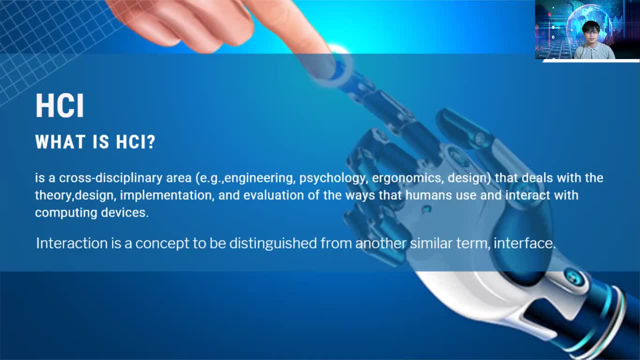 are going to be talking about the different standards you know in the next chapter. So I hope you guys have get the idea what a human-computer interaction is. So again, it basically focuses on the interface between the computers and the user. 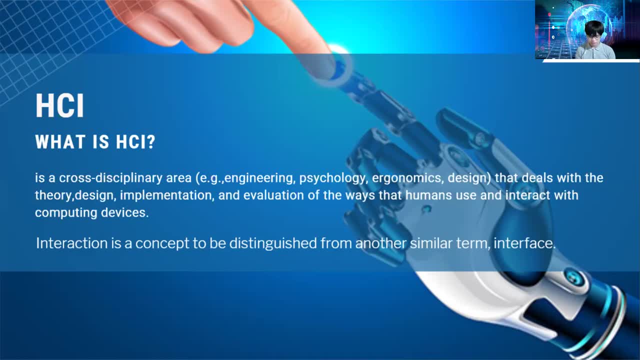 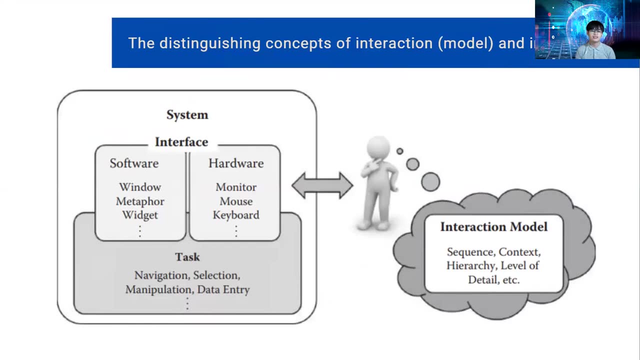 as the user or the people. Next, the distinguishing concept of interaction model and interface. So when we say interaction model, it's actually. it involves the sequence, the context, the hierarchy, the level of data and a lot more. When we say interaction, it actually it involves software & hardware. 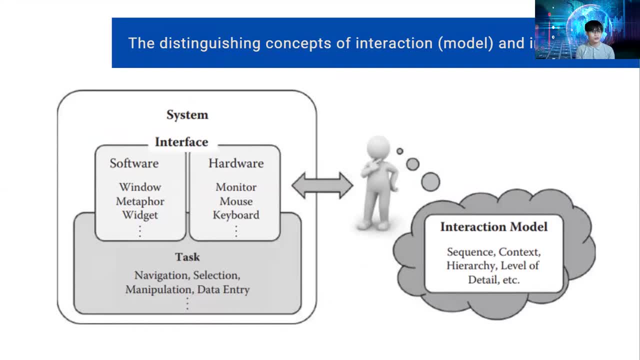 It would be very hard to interact without the software and hardware. Software means, I believe, Premina Nimimisha exist, or you always hear about software. So when you say software it involves window meta for fidgets, those applications that you have seen in. 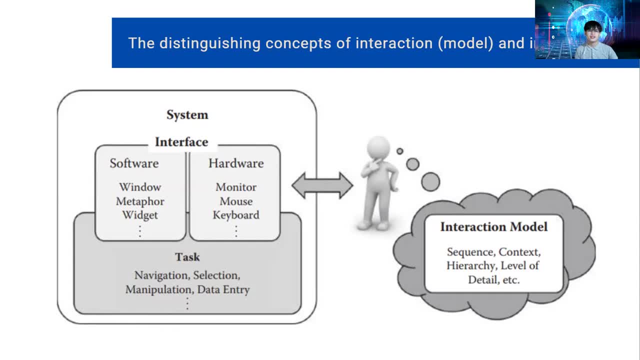 your hundred phones in your computers, anything that is installed in your computers. so this is software: the icons, the interfaces that you're seeing, you know, arrows in the borders and etc. okay, and this where in the software? okay, as for the hardware, of course, these are the tangible materials. very, 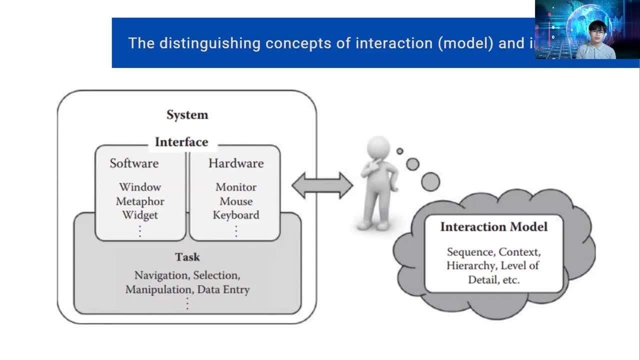 understandable. so it involves monitor, mouse, keyboard system, unit, cord. okay. and when you, when there is an interaction now between the software and in hardware, there is what we call the task. so I believe you know what task is all about. so when you actually navigate, so when you select, when you manipulate and there, 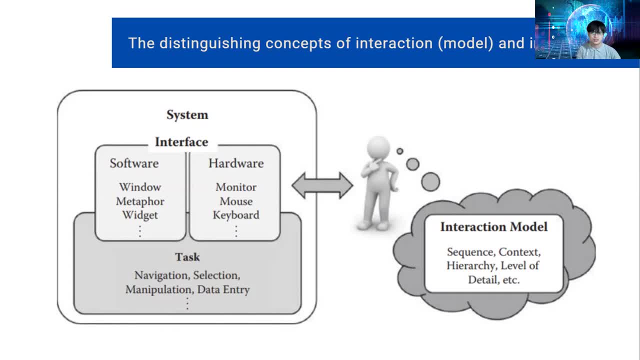 is an encoding it entry. there is an interaction between the software and between you and then the computing device, that is, you are creating a task. so this is how you distinguish, actually the interface and then the interaction model. so I hope, you hope, you hope you've got some idea. 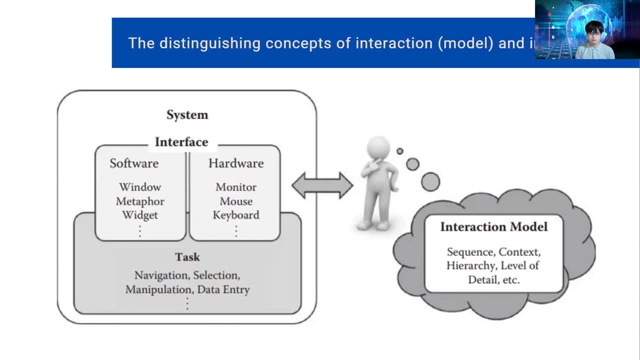 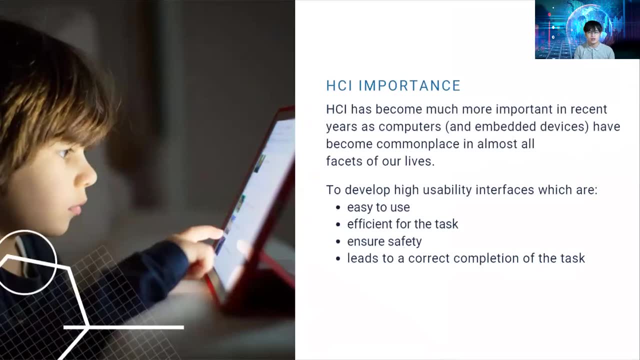 about, about this term, okay next. okay, we proceed with the importance of HCI. so why do we need HCI? to learn about this. HCI the computer, a human computer interaction. so HCI has become more important in recent years as computers and embedded devices have become commonplace in almost all facets of our life. I hope this is really clear. 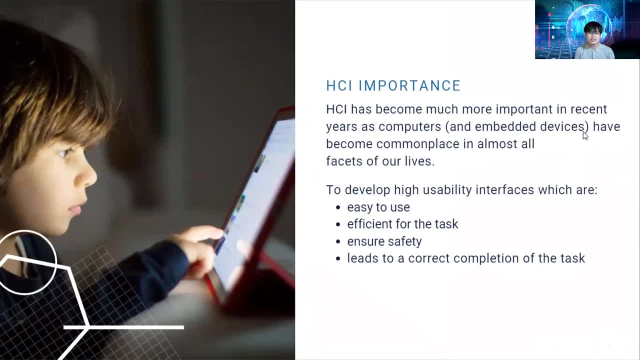 for you guys that we really need to study HCI again. it's become the commonplace in almost all facets of our lives, especially today, especially that we are doing a flexible online learning. okay, so without computers, without any computing devices, without the Android phone, your laptop, then it would not be possible. okay, and also, why do we need to learn about HCI? 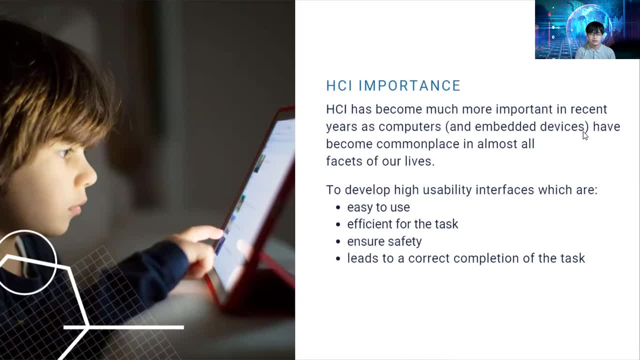 is for us to be able to help develop a high usability interface or systems- systems which, as I said in my previous video, there are many types of HCI that we need to learn about- and for all of us to be able to help develop a high usability interface or systems systems which are high usability interfaces or systems which are. 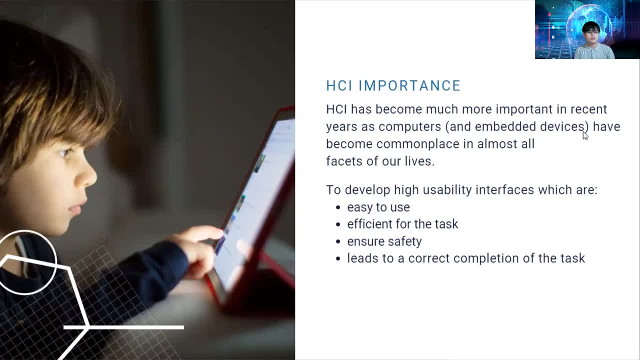 are easy to use, systems which are, which are efficient for the task. it ensures safety and leads to a quick completion of the task. a system can, of course, solve the problem right. so that is why HCI, or human-computer interaction, is very important now, because if we're gonna help- not help solve problems- and yeah- 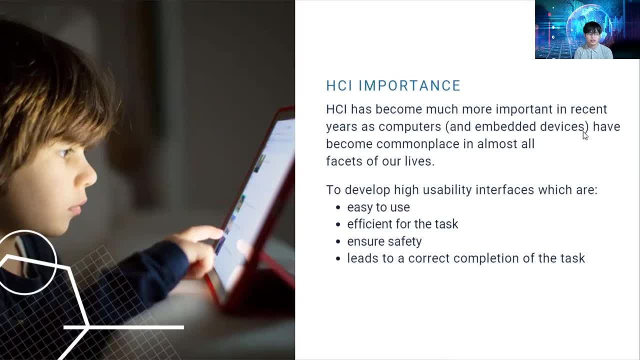 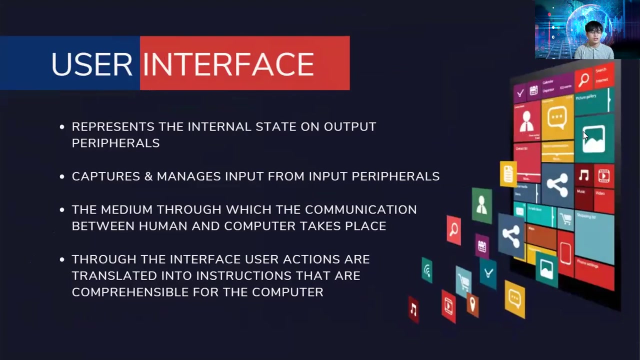 okay, so we hope you understand why do we need to learn about HCI, why do we need to be enthusiastic in terms of technologies? because, as technology students, as technology students, you must and you should be able to, of course, design your own software. okay, so let's understand. know what user interface is all about a UI. so I 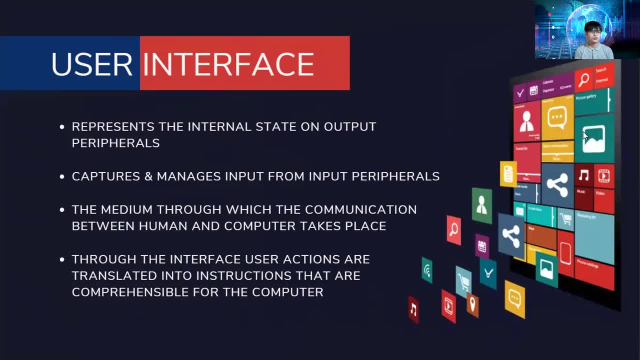 believe you heard about UI and UX, but you don't have any idea what truly UI and UX means. so, user interface: it represents the internal state and output peripherals. it captures and manages input from input peripherals. it captures and manages input from input peripherals. it captures and manages input from input peripherals. 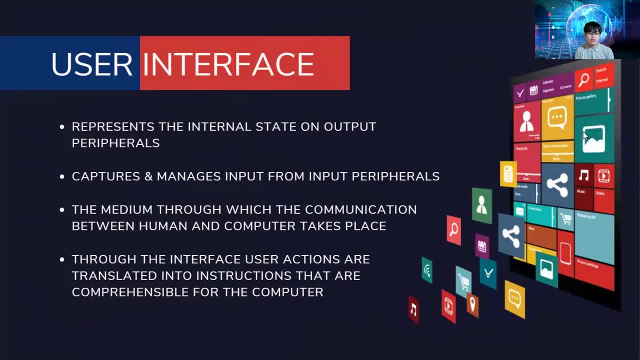 so you can easily make a lot of a different outcomes based on the, the, the internal state of the output peripherals it captures in, manages the medium through which the communication between human and computer takes place, and through the interface, user actions are translated into instructions that are comprehensible for the computer. So the user interface is where the human 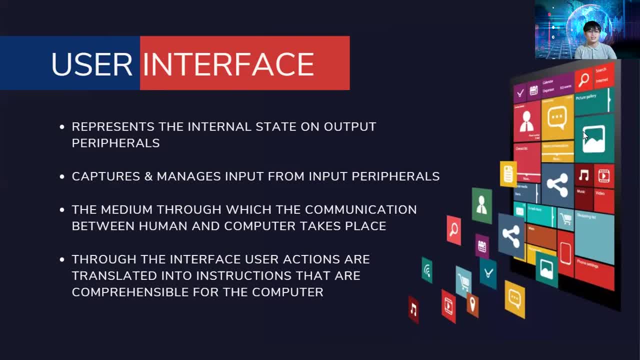 and computer takes place. This kind of starts in creating a task, in manipulating what's in the software or what's in the system, right. So again through the user interface, the user actions are translated into instructions. So for example, you click a button, you click a login button, so that click will be. 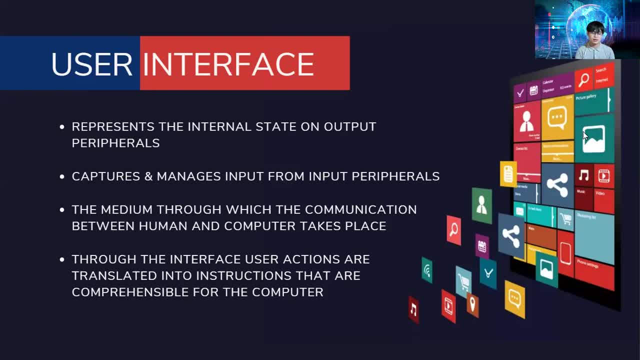 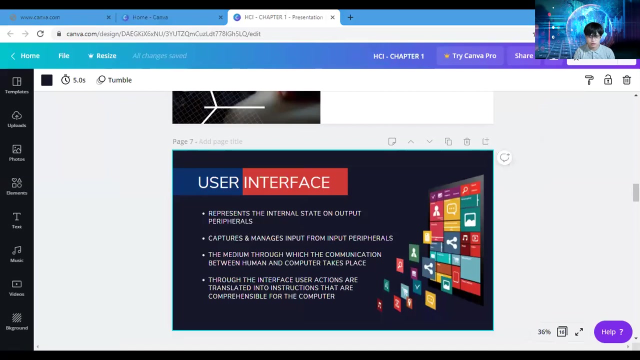 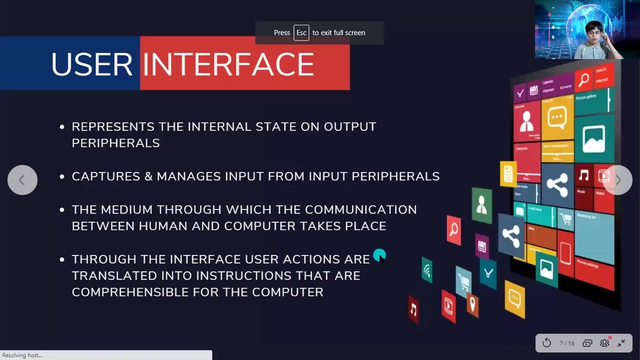 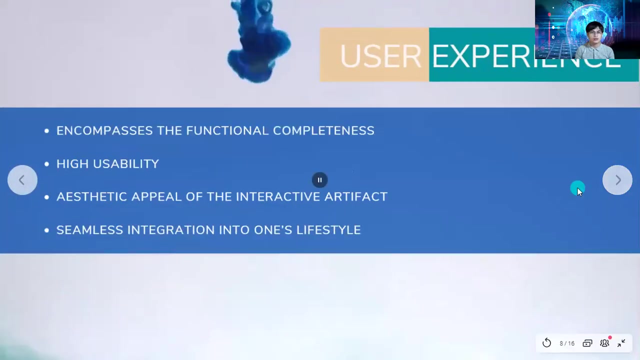 translated into computer language. So what you've seen, what you've seen in the, in the interface, is Okay. so that's it. That is user interface. Next would be the user experience. So what is UX, A user experience? It actually encompasses the functional completeness. 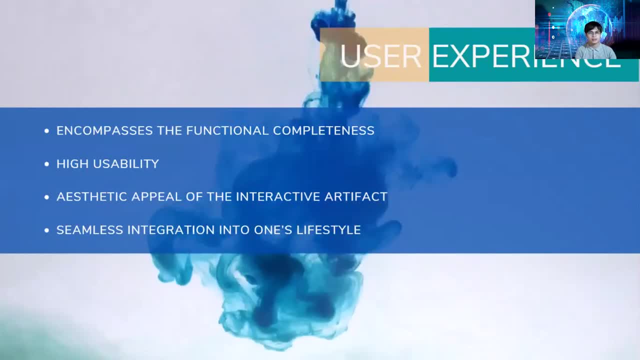 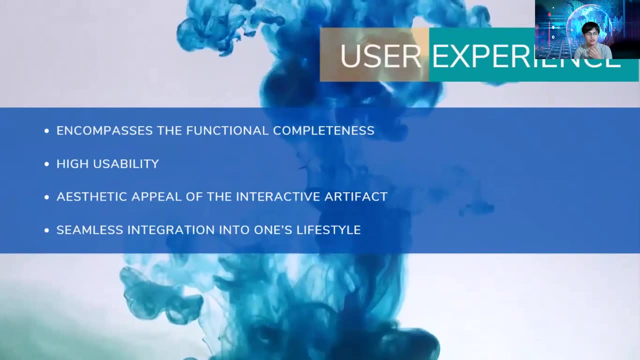 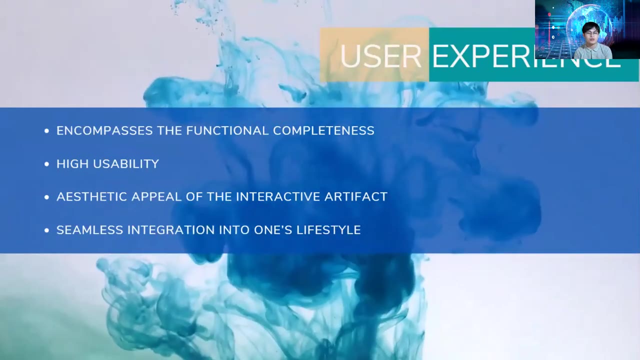 it involves high usability and aesthetic feel of the interactive artifact. it is a seamless integration into one site we use. a user experience is this: It involves all functional completeness organizations. So of course, from the transition itself, the user experience that involves that all functional completeness of the system. So let's talk about that. First user experience. it involves completion. 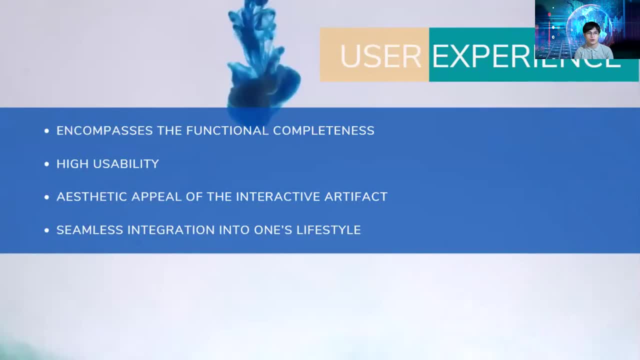 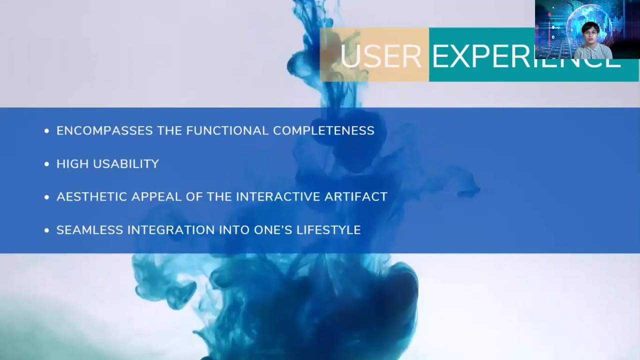 with all functional completeness of the system. So of course, from the traffic itself, user experience, What we've seen in the transit itself, user experience now how the user will going to use the system or what will be the experience now of the user if he used that kind of software. so it's very important. 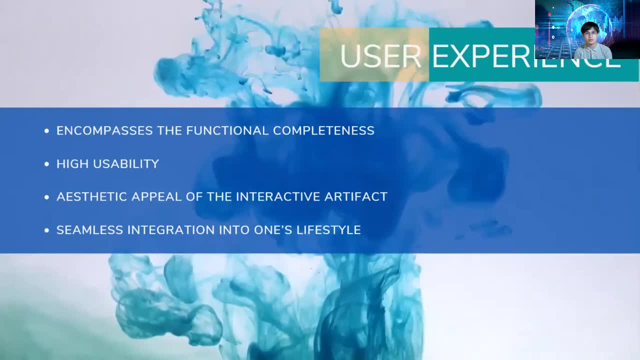 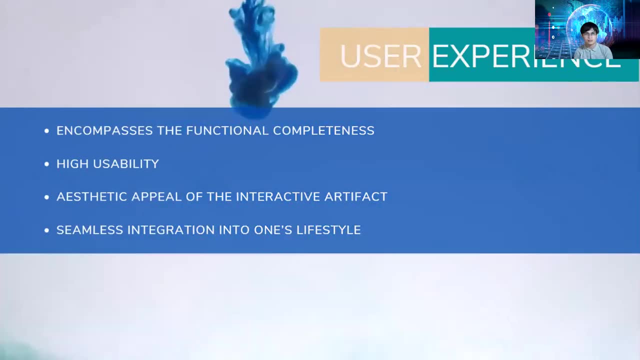 you should clearly understand what ui into it means. so when, when creating a system, when creating a software, the ui and ux must be really, really good. you know for your system to be, you know for your application to be, of course, a success, so it it should be, you know, pleasing. 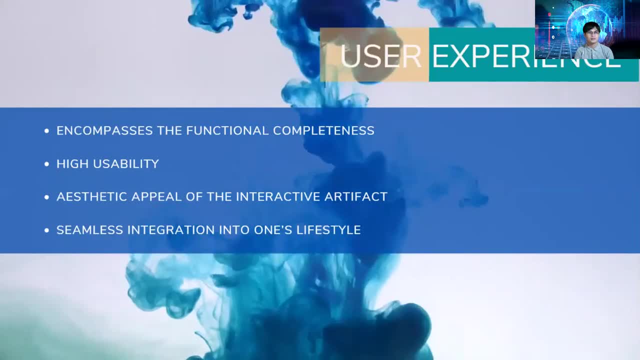 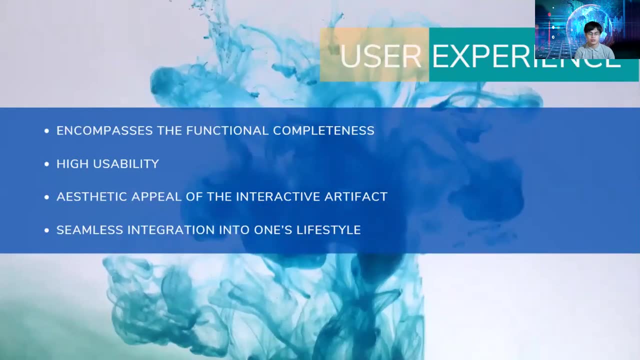 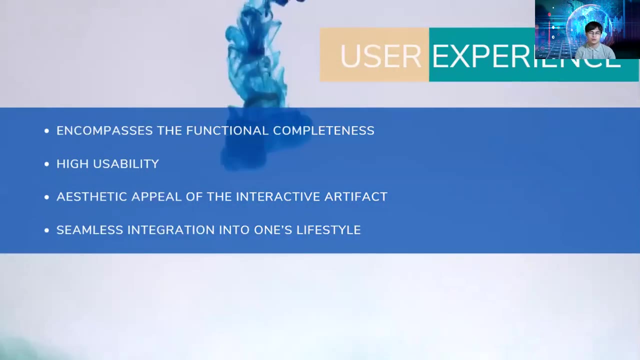 of the eye should be um, easy to use and use of all the applications. but don't worry guys, we're gonna be talking about it later on the next chapter. so there would be a lot of standards that you need to follow, follow in order for you to create your own uh, your own applications, ui and ux designs to be 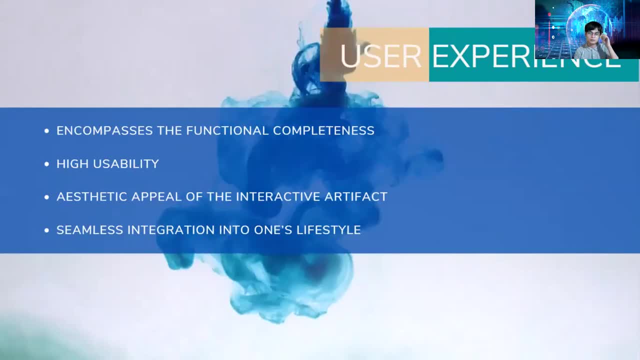 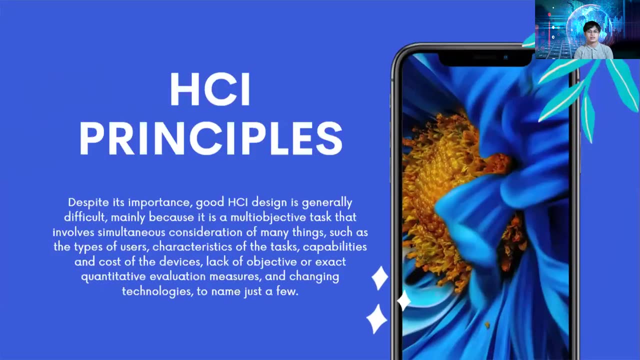 more you know more, um, really really good, okay, next, okay, next topic is the hci principles. what are the different principles of human computer interaction? so, despite its importance, good hci design is generally different. indeed, you know, it's not just design without, without even knowing what are these different? 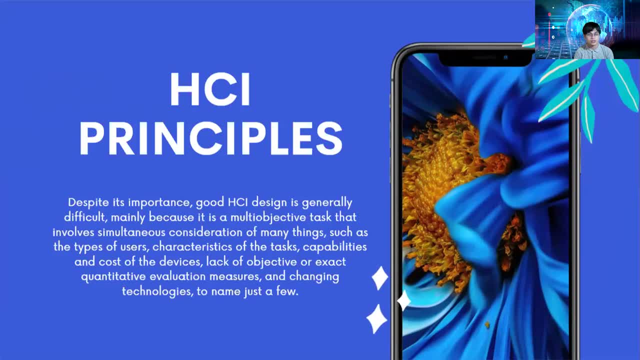 principles, mainly because it is multi-objective task and that involves simultaneous consideration of many things. so there are a lot of things that you must consider, such as the type of user who are going to use your application. is it is the application for the kids or is it for the adult? 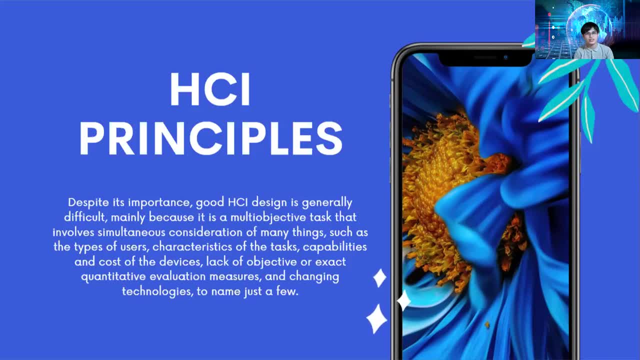 and the characteristics of the task. so what are the different tasks? what are the different features that your application will going to do you know on how to how it will solve the problem. it kept the capabilities and cost of the devices. it's very important. the cost lack of objectives. 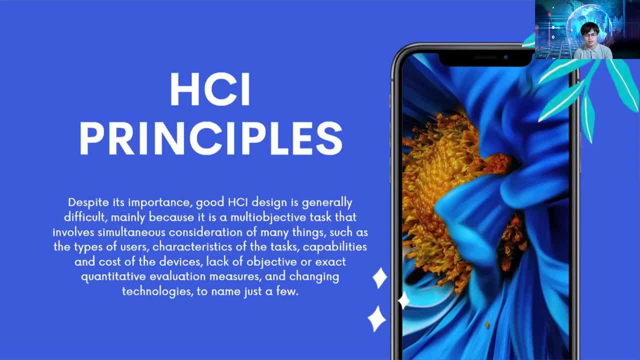 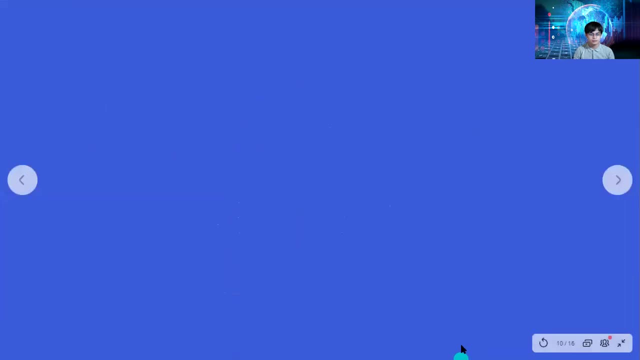 what is your objective? what is the purpose of the system or of the audit software for exact quantity, and of the system and the environment? I think the the primary function of the hci is to. if you're working with a user, it's important to know what are the exclusive evaluation measures. 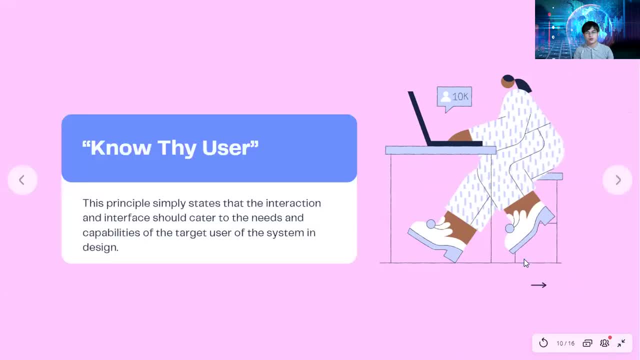 and changing technologies, to name a few. so let's start with the first principle. okay, know the user, know your user. this principle states that the interaction and interface in the design. so it's very important that before creating a system, you should be able to target, know who will be, who will be your user or who are going to use your system, because it would be very 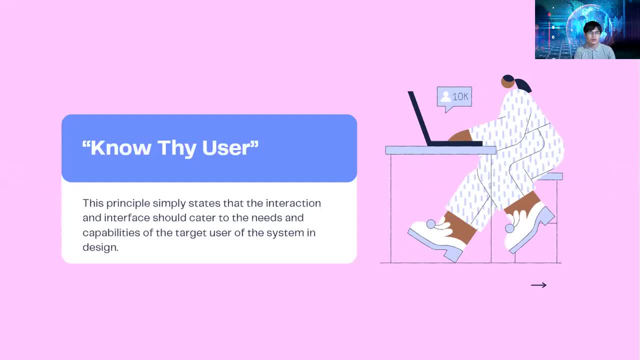 hard to design, to create software without knowing who is your targeted user. okay, so, for example, you develop an online shopping system, an online shopping that is good for a student, that is good for senior citizens, and then when the senior citizens use that kind of online shopping application, then the senior citizen cannot really understand or doesn't know how to use your. 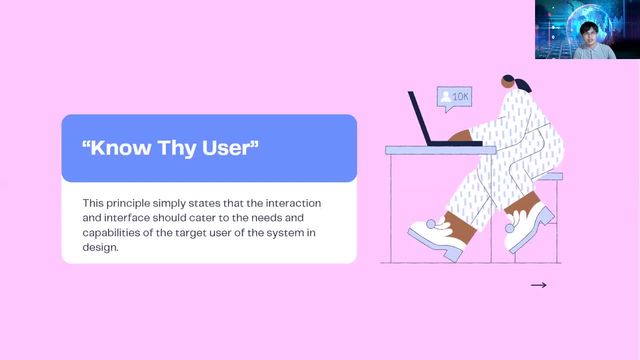 software because you you've developed or you design it, just you know, for for their students, something like those things. it's very important they should understand who your target user is. okay, is your application for the kids only? no, is it for the teens only. is it for the adults? so something like those things. 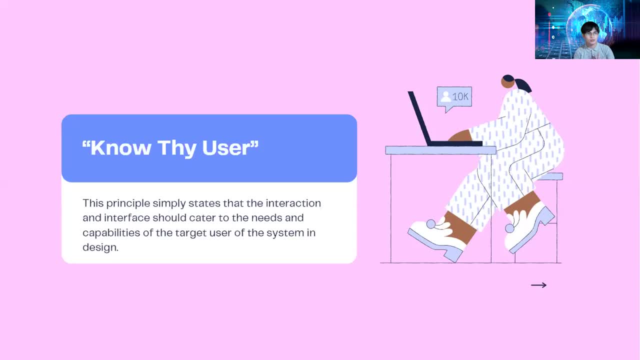 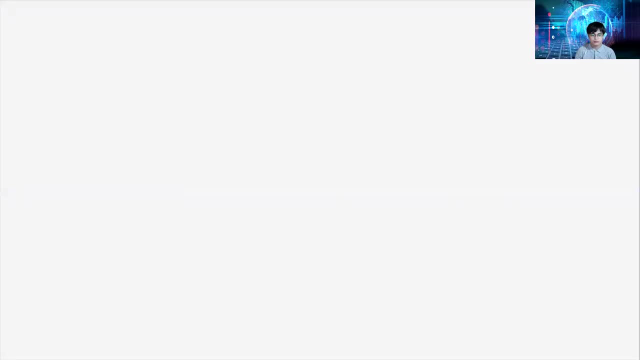 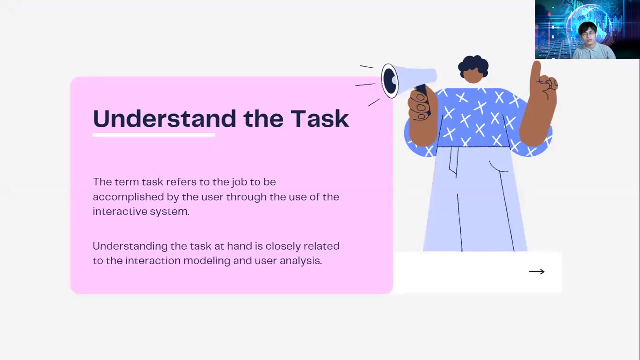 okay, that's one principle again: you must know your user before creating your software, before creating your system. next is: understand the task. okay, understand the task. what are the different tasks in the system? okay, so the third task refers to the job to be accomplished by the user through the use of the interaction system. so what are the? 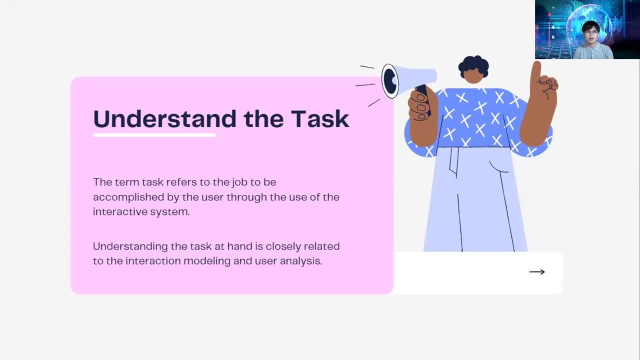 different features of your system. okay, for example, if the user is going to click this icon, what will gonna happen? now, if the user is gonna click the login button? well, the user will be navigated to the dashboard, where the user will be navigated to his profile, something like those things. so you should. 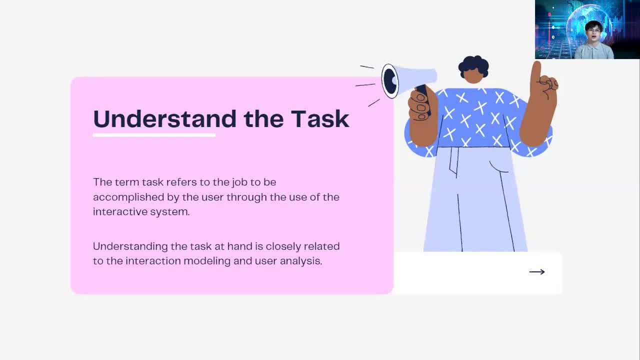 must understand. now you should have this um checklist or or different, you know, project details of the system in which you have um already determined the different features, different tasks that you're going to do, or the jobs that the system will. we're going to, we're going to gonna detail some um. why makita's user? okay, understanding the task at hand is closely. 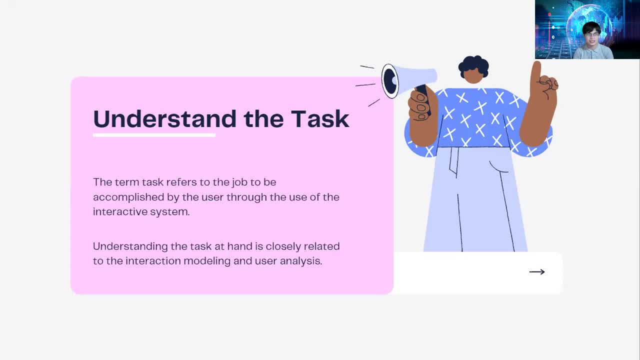 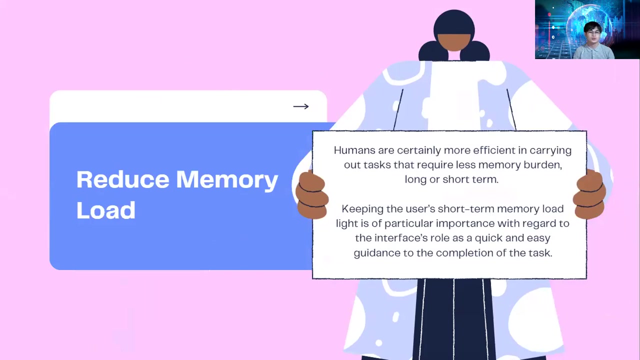 related to the interaction modeling and user analysis. so, as a developer of the system, if you put yourself as the user, always no, and then yeah, okay, okay, reduce memory load. so when you say reduce memory load, humans are certainly more efficient in carrying out tasks. that requires less memory burden, long or short term, keeping the users their 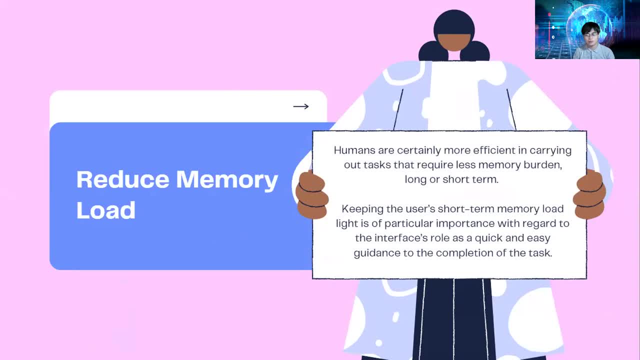 memory load. memory load light is of particular importance with regard to the interfaces tools, as quick and easy guidance to the completion of the task. of course, as a human being, we need to be aware of the tasks that we are carrying out. we need to know how to use the systems we're using. are they efficient? are they? 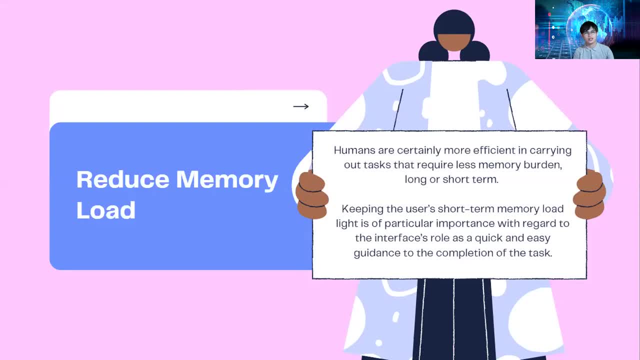 effective, are they reliable, are they safe? so, for example, if you log in to that application, we want to log in, we want that. so, um, as you may have noticed that, if, if that kind of application doesn't have a good memory load, and then you are gonna have to build, so we're going to install this application. 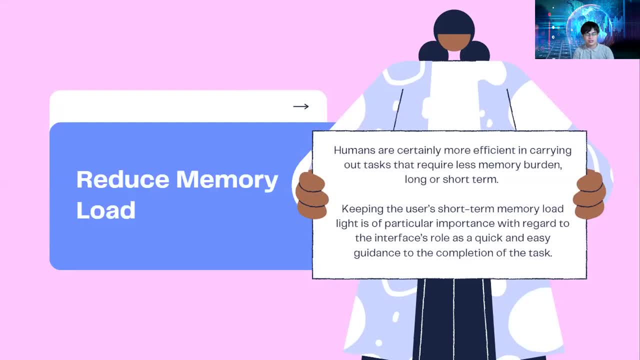 we don't use that application. So it's very important that when you design a system, you should know this kind of principle, Know that your application must be in a good performance where, if there are tasks that the users were going to do, it would be you know. 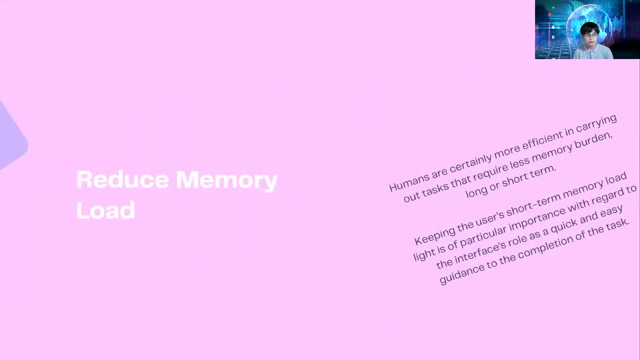 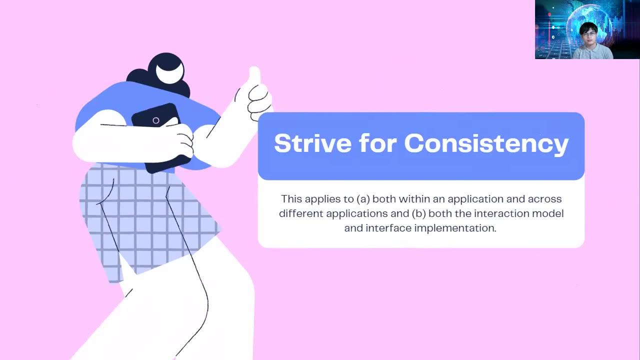 something like those things. It must be quick and easy. Next, strive for consistency. As for the consistency, this applies to both within an application and across different applications, and both the interaction model and interface implementation. So there should be a consistency. It must be consistent If your interaction model 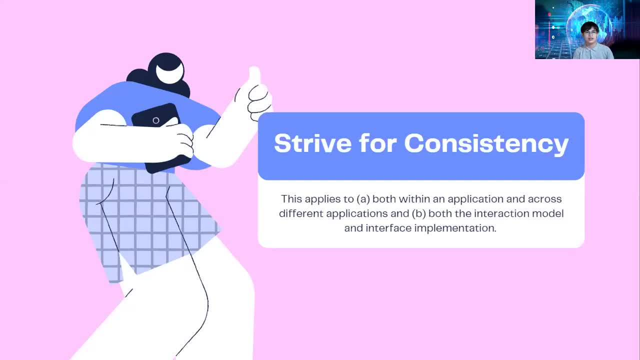 is, you can define it like this, like that, then the interface implementation should be the same with your interaction model. So don't worry, because, as for the consistency, you will be able to discuss further later and how are we going to apply it to our system. 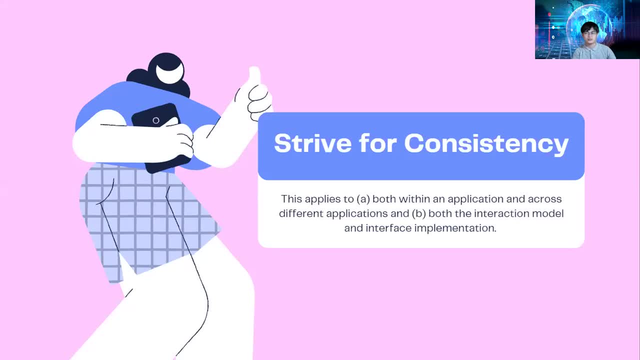 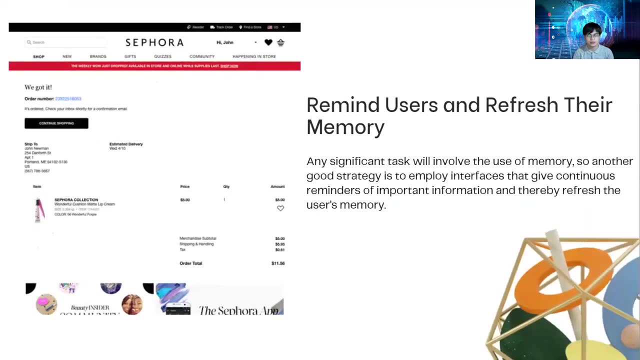 So it must be consistent: the interaction model and the interface implementation. So, yeah, Next principle is remind users and refresh their memory. Okay, what does it mean? Any significant task will involve? any significant task will involve the use of memory. Okay, so another good strategy is to employ interfaces that 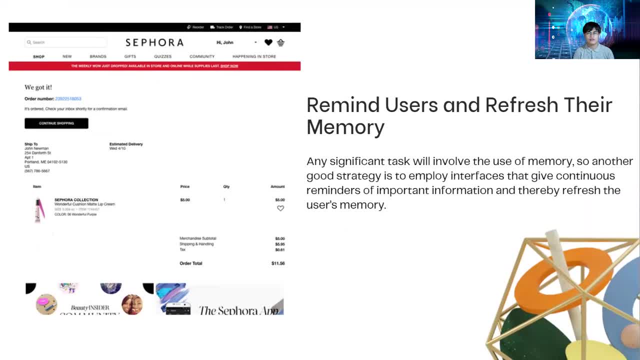 give continuous reminders of important information and thereby refresh the user's memory. Okay, so let's say, for example, you have developed a shopping application. As for the shopping application, we know that the user will gonna add products. you know, add products to the cart And by the time of the 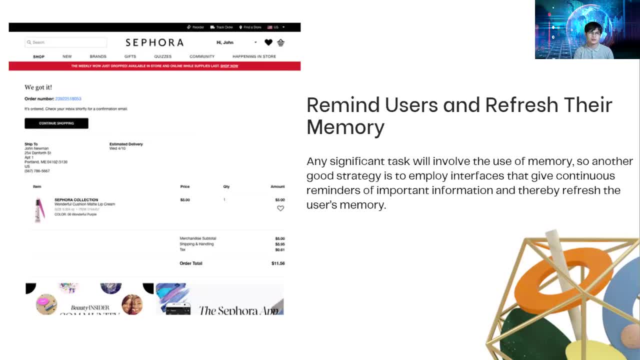 checkout, the user will ask himself: so what are the different products that he added, Or he added, to his cart? So it's very important, since, after the checkout, there should be this confirmation page where the user will be to view the different products that he or she ordered, So something like this. Okay, so we must. 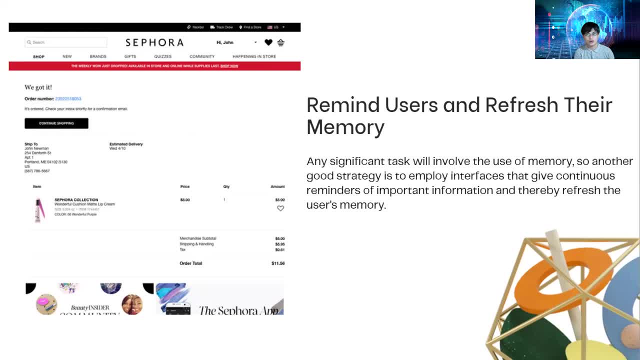 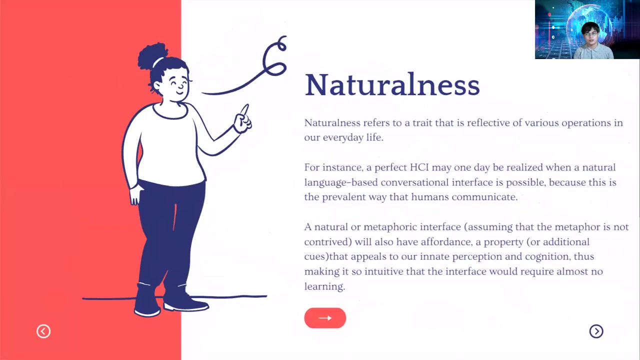 always remind the users: what, how, what did he do to the system? Essentially? Yeah, that's what I wanted to add, Andrew Adelman, I've said in the shapping application. Next and last principle of human-computer interaction is naturalness. Naturalness refers to a trait that is reflective of various operations in our everyday. 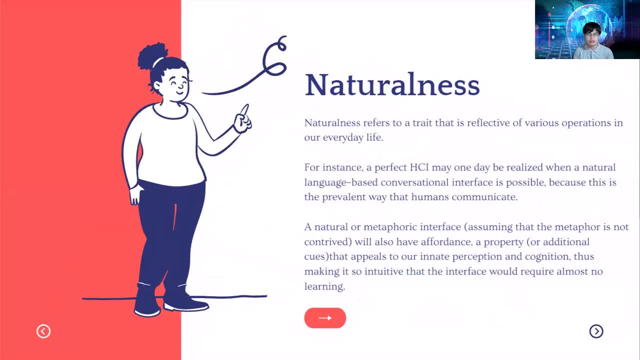 life. For instance, a perfect HCI may one day be realized when a natural language-based conversational interface is possible, because this is the prevalent way that humans communicate. A natural or metaphoric interface- assuming that the metaphor is not contrived- will also 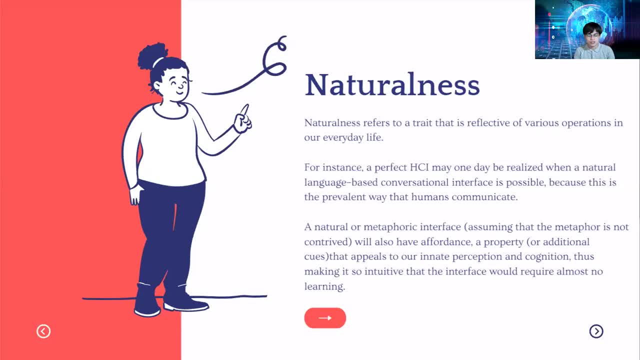 have affordance, a property or additional cues. that appeals to our innate perception and cognition, thus making it so intuitive that the interface would require almost no learning. So for you to easily understand what naturalness is, your application must be user-friendly. 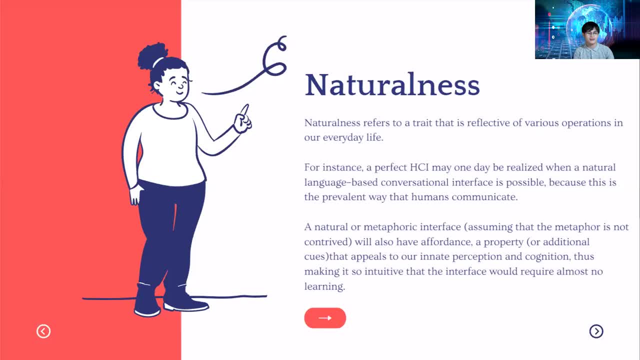 It must be simple as possible. quick and easy to navigate, So it would actually require almost no learning, So the user will no longer be able to have a lot of trainings in order for him or her to use this system. It should be simple, For example, Facebook. 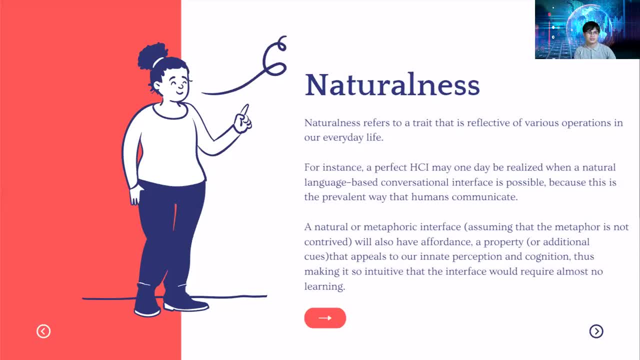 Everyone can use Facebook, Even if the young kids know. there's no more training. just help them create their accounts, then log into Facebook, then do their thing, So something like those things. It should be quick and easy. It should be user-friendly, Okay So. 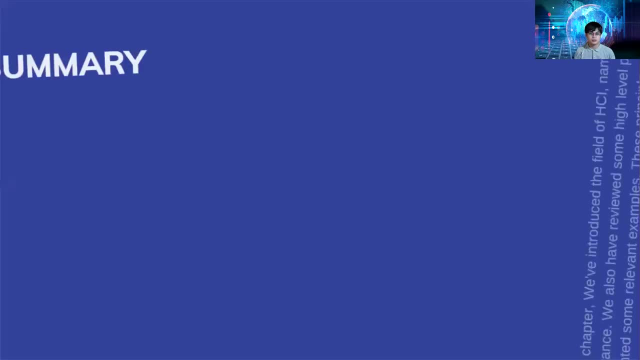 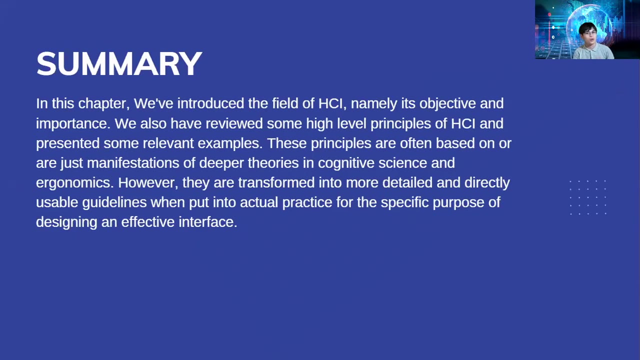 that is the principle of HCI. Okay, So I think that would be all for this video. We have entered the end of the session. Thank you, Thank you. When we first started with this talk, we were able to learn what HCI means. 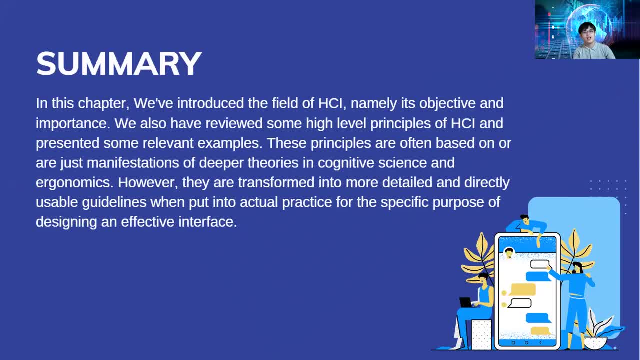 It's just that HCI Intel is basically an interface and it introduces what HCI means. why is it important that we need to learn it, why do we need to design in the interface And also what are the different principles that we need to consider before waiting for? 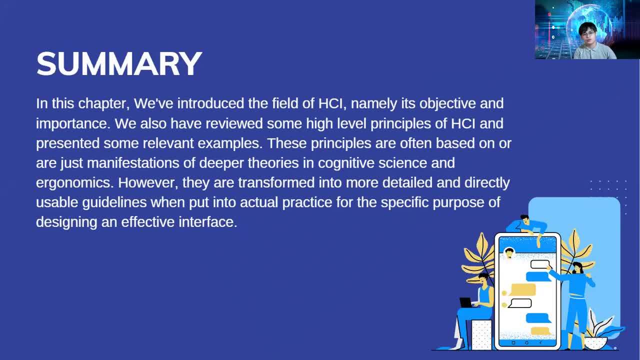 HCI. Okay, So as far as the summary. in this chapter we've introduced the field of HCI, namely its objectives and importance. These principles are often based on or are just manifestations of different theories in cognitive science and ergonomics. 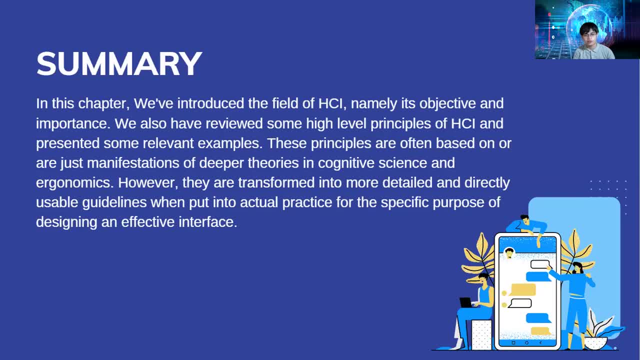 However, they are transformed into more detailed, indirectly usable guidelines when put into actual practice for the specific purpose of designing an effective interface. So in the next chapters we will be talking and doing about how to design a really really good and effective interface. 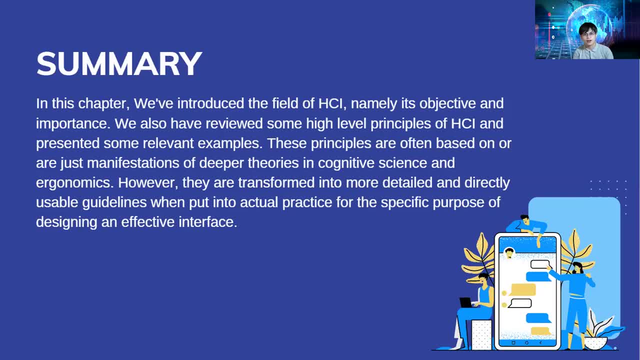 So I hope you guys have learned something. If I'm too fast, just review the video and review the slides. The PDF also will be available for you And if you have any questions, just feel free to reach me out, and that's all. 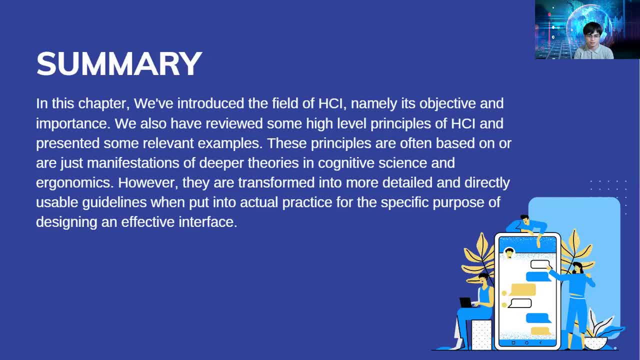 So that would be all. Thank you so much. Thank you for watching.